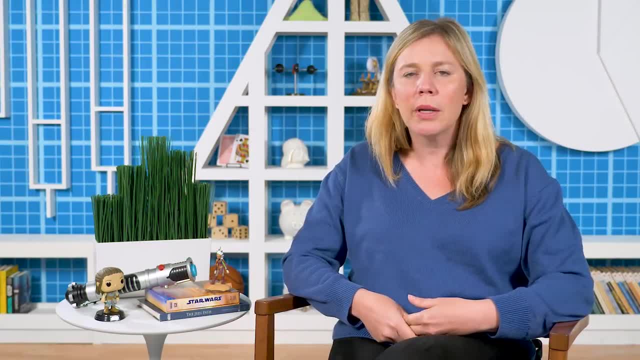 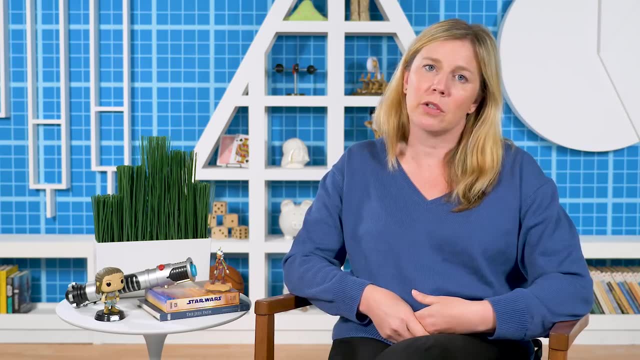 of A and B. For example, when you're out to lunch, your sister mentions that she has a friend who has breast cancer, But she doesn't say much else. You recently saw a documentary about males with breast cancer. Because it's so fresh in your mind, you wonder if your sister's friend is a male. 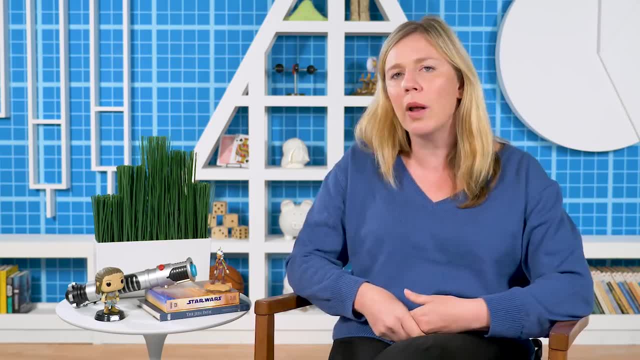 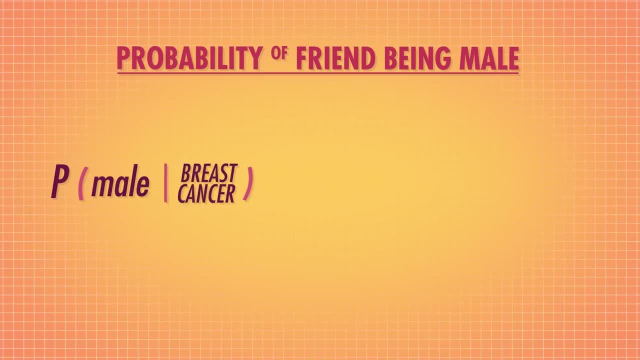 Your gut feeling is that it's not likely they're male. But let's quantify it. You want to know the probability that your sister's friend is male, given that you know that friend has breast cancer. Using Bayes' Theorem, we can calculate this probability. 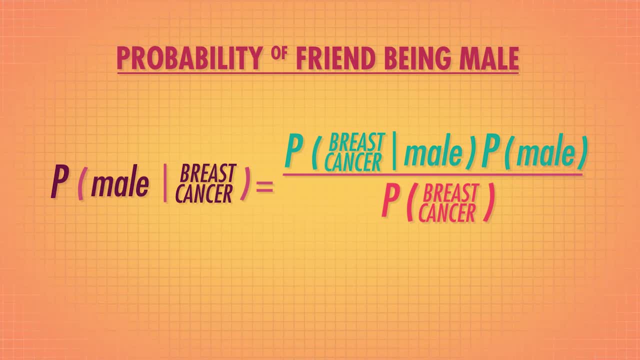 The probability of being male, given you have breast cancer, is equal to the probability of having breast cancer given that you are male… times B times the probability of being male divided by the probability of having breast cancer. Thanks to government health agencies, we know many of these statistics. 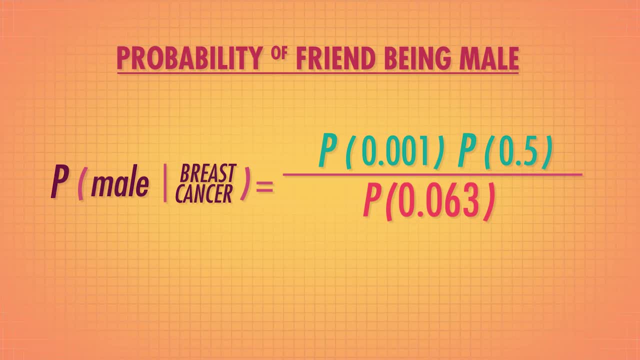 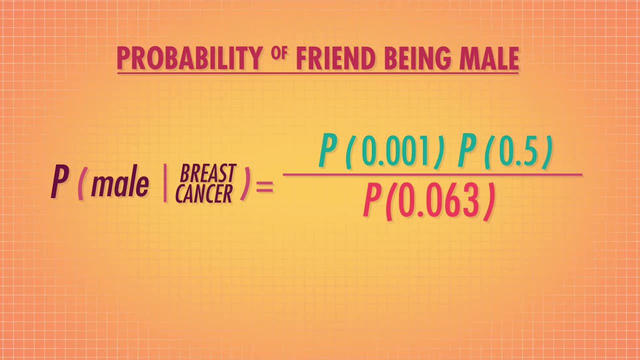 The probability of getting breast cancer, given that you're male, is 0.001.. And we'll assume the probability of being male is 0.5.. The overall probability of getting breast cancer is 0.063.. Armed with your facts, you calculate. the probability that your sister's friend is male is only. 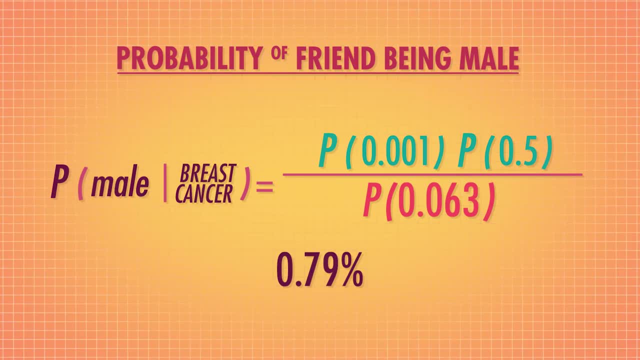 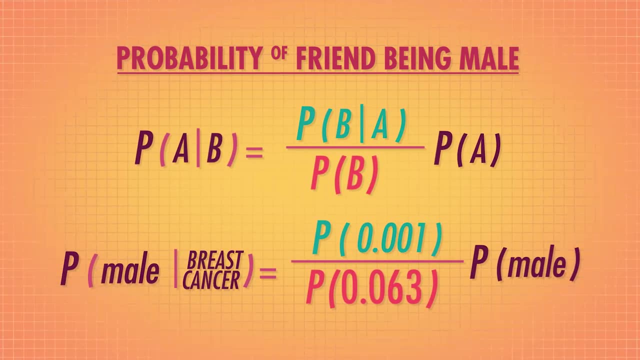 about 0.79%, So not very likely, but maybe more likely than you would have anticipated. If we rearrange Bayes' theorem slightly, we can see that it allows us to update our beliefs based on new information. When we use Bayes' theorem, what we're really doing was updating our belief that. 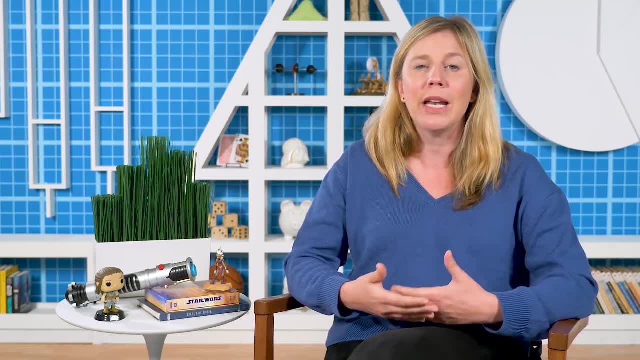 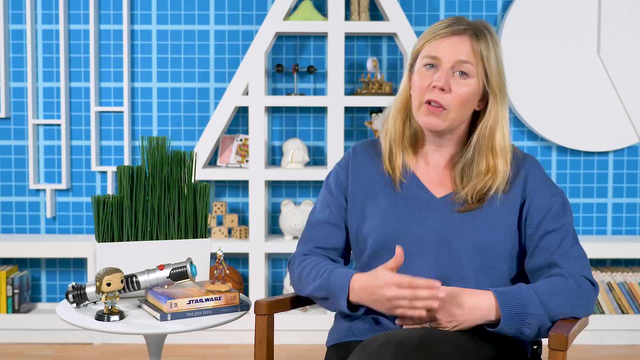 a person was male, probably about 50-50 odds if we don't know anything else about them. with the new information that they had breast cancer, This new information changed our belief. We went from a 50% chance to about a 0.79% chance. 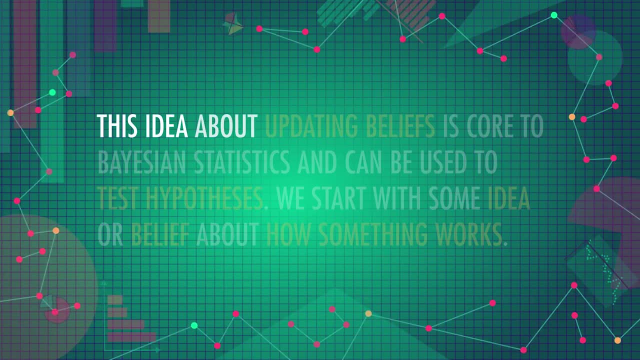 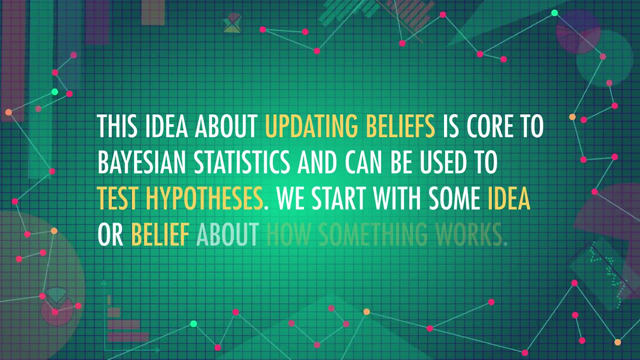 Just by taking into account this new information. This idea about updating beliefs is core to Bayesian statistics and can be used to test hypotheses. We start with some idea or belief about how something works. For example, you set your friend Maria up on a blind date. 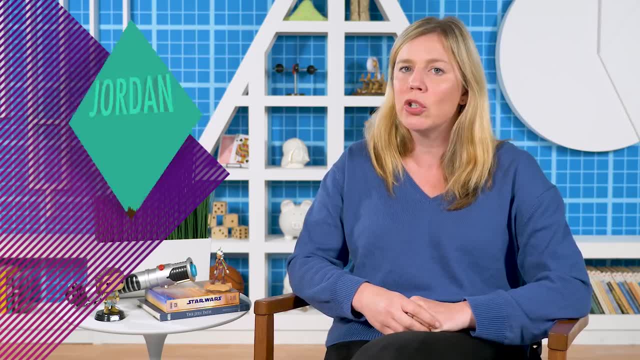 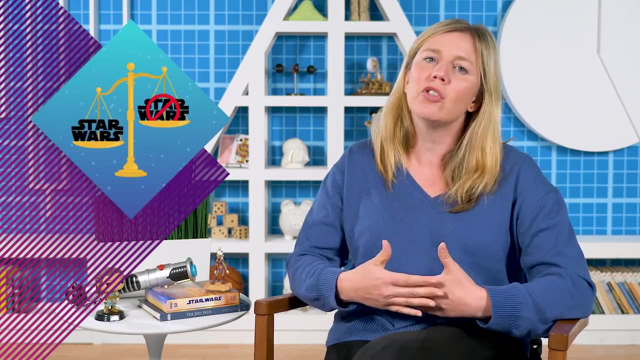 Maria is excited but nervous, and on her way to the coffee shop to meet her blind date, Jordan, she wonders whether he shares her love of Star Wars. From her experience meeting people in the city, she believes that in general, there are slightly more Star Wars fans than non-fans. 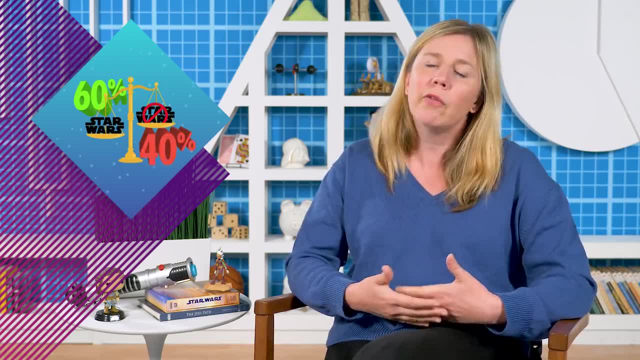 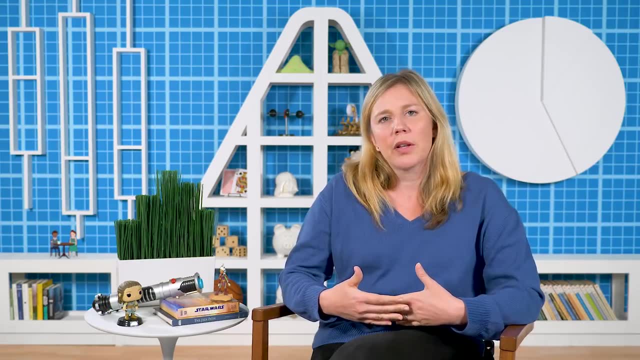 There's a 60% chance that a given person is a Star Wars fan and a 40% chance they're not, which means she thinks it's one and a half times more likely that someone's a fan. When Maria arrives at the coffee shop, she and Jordan do the normal first date small. 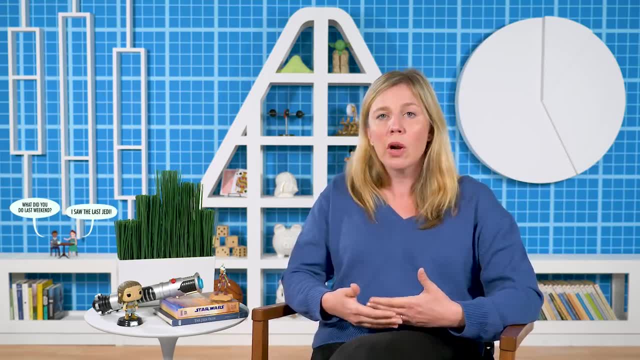 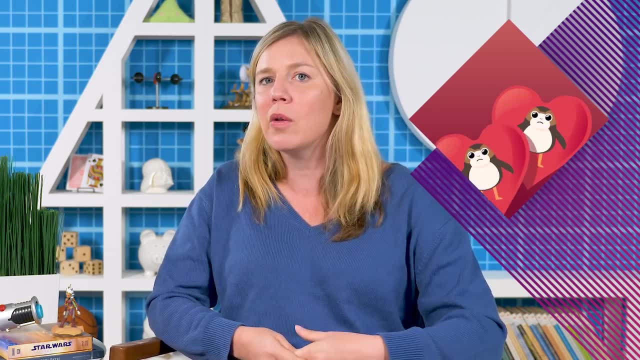 talk. He asks her what she did last weekend and she told him she saw the new Star Wars movie. Jordan says he did too. After hearing this, Maria feels like it's more likely that she might have met her poor, gloving soulmate. 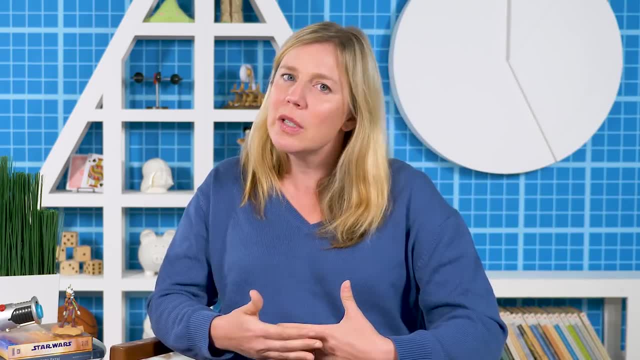 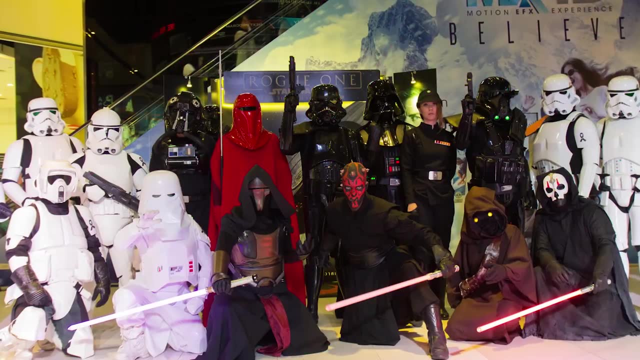 She knows that not everyone who's seen Star Wars is a fan, but she can use the fact that Jordan has seen it to update her belief about whether or not he's one. Maria knows that the probability of having seen the last Star Wars movie, given that 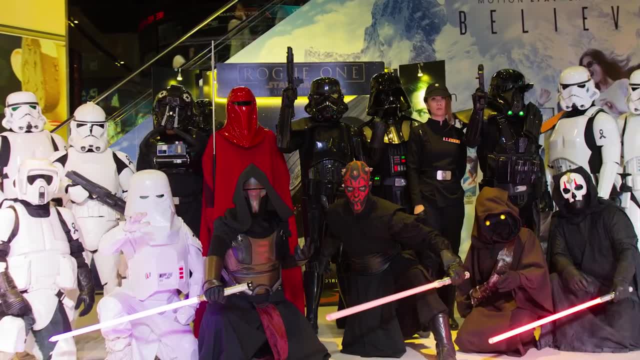 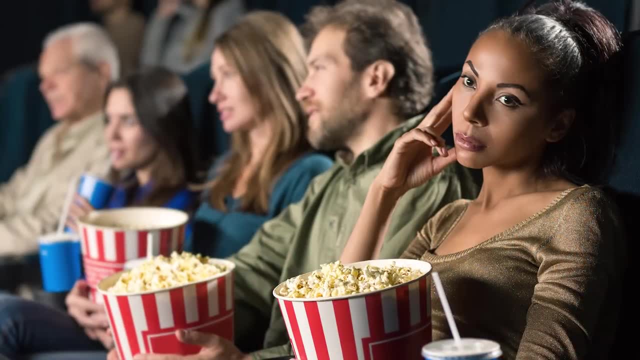 you're a fan is 0.99, since pretty much all fans rushed to see the movie. But not everyone who went to see the movie were fans. Some were just curious and others were dragged by family or friends to see it. 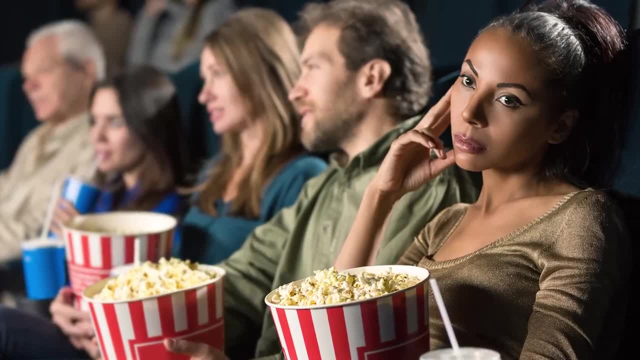 She thinks that the approximate probability of having seen the movie, given that you're not a fan, is 0.5, since some fans went to see it. For more information on what happened, please visit our websitecom. fans went to see it. 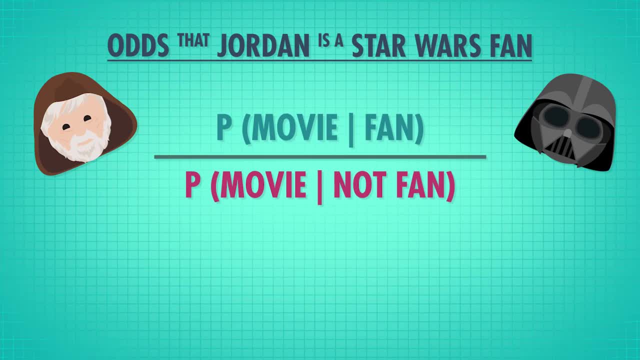 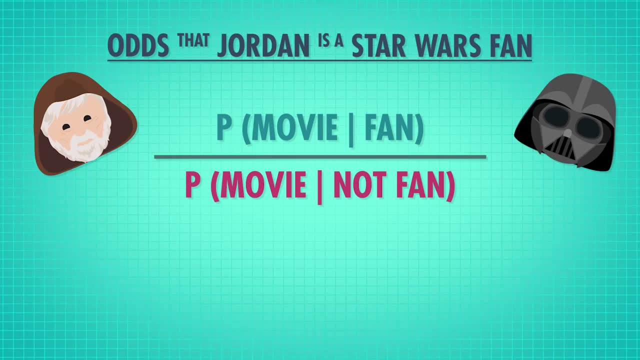 Maria can use the ratio of these two probabilities- probability of movie given fan and probability of movie given not fan- to see which hypothesis is more probable, given that we know Jordan saw the movie. Based on Maria's quick calculations, this new information means that it's now 1.98. 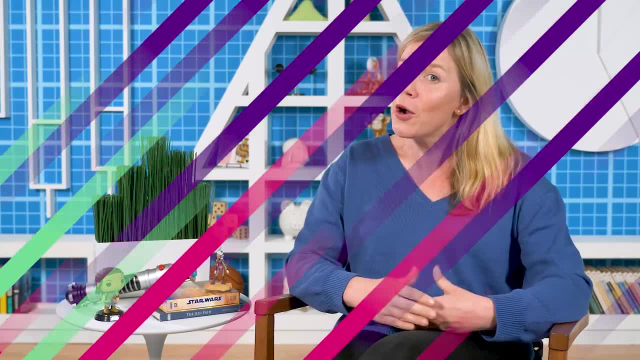 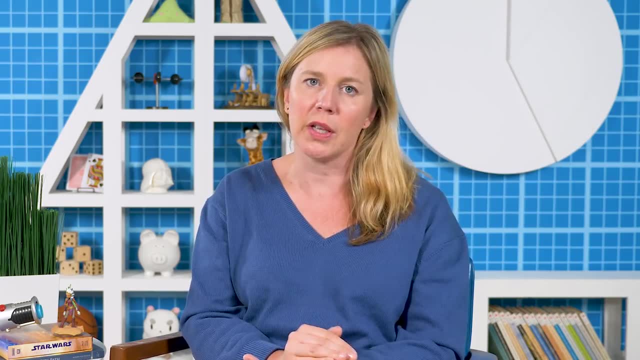 times more likely that Jordan is a Star Wars fan than not, Her heart starts beating a little faster. The ratio of the probability of our information under one hypothesis that he's a fan compared to another that he's not a fan is called a Bayes factor. 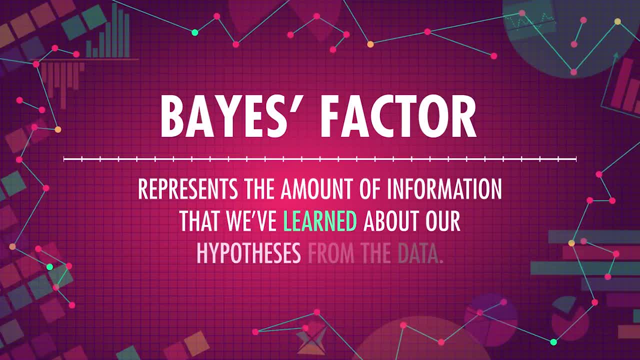 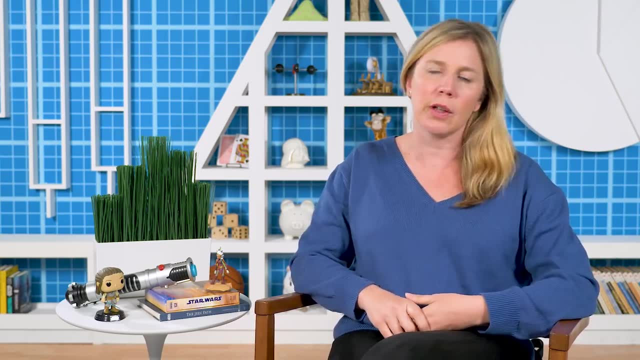 It represents the amount of information that we've learned about our hypotheses from the data. Maria can use it to update her previous belief or prior odds that it's 1.5 times more likely that Jordan is a fellow Star Wars fan. All she has to do is multiply her prior beliefs- the ones she held before she had any new information. 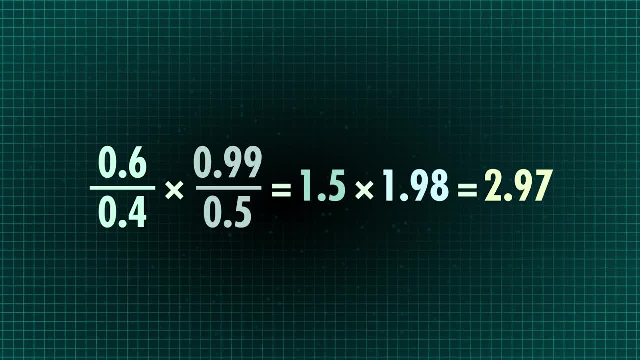 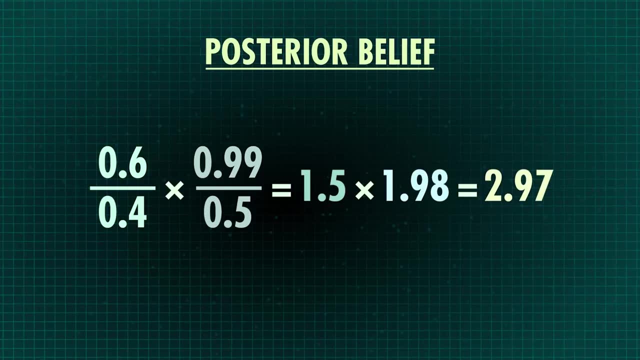 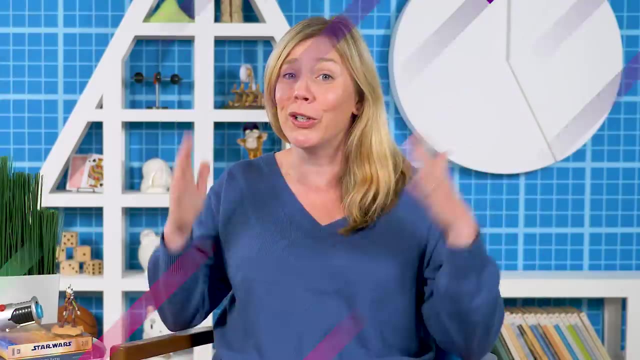 by the Bayes factor, which tells her how much to change her belief now that she has some evidence. The resulting belief is called her posterior belief, In this case 2.97. And she can continue to incorporate new information. When Jordan says his dog is named Anakin, she can again update her beliefs. 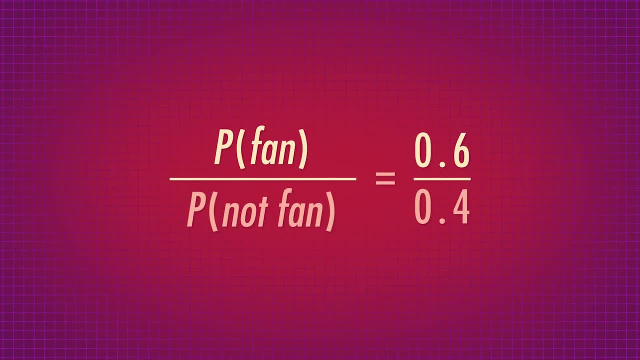 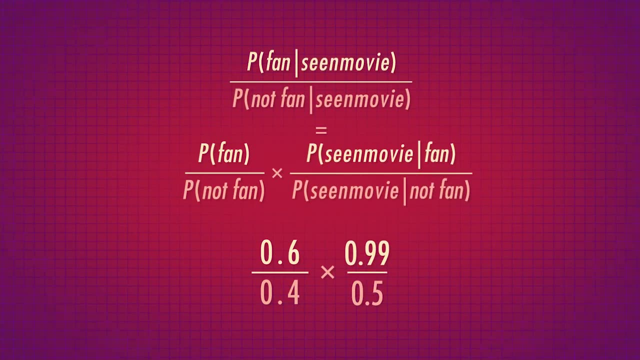 Or just ask Mathematically. we took Maria's prior belief and updated it with our Bayes factor, which told us how much data Jordan seeing the new Star Wars movie should change her beliefs about his fanhood. This is a very simple example of how we can use Bayesian hypothesis testing to compare. 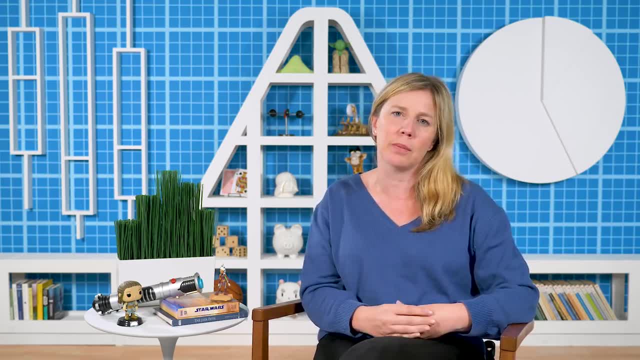 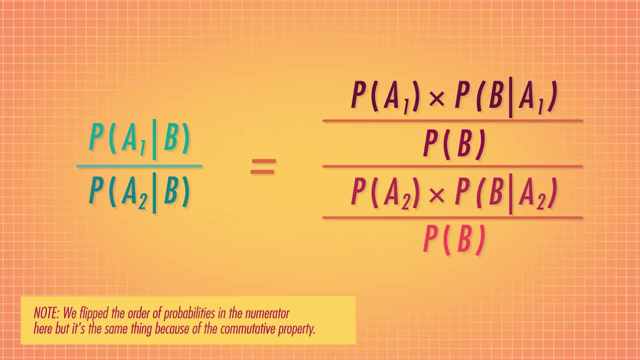 the probabilities of different hypotheses based on the data we observe. But this doesn't look exactly like the Bayes Theorem that we saw at the beginning. That's because, instead of looking at the probability of one hypothesis given the data, we're looking at the ratio of two hypotheses. 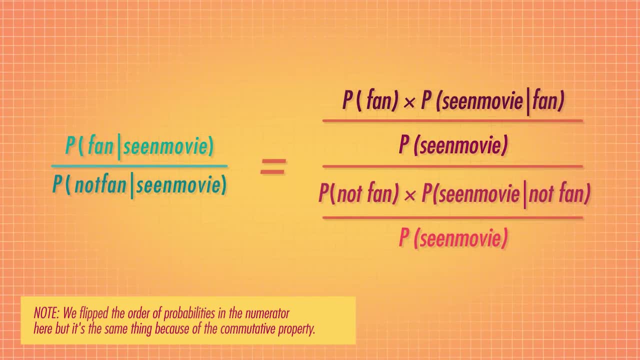 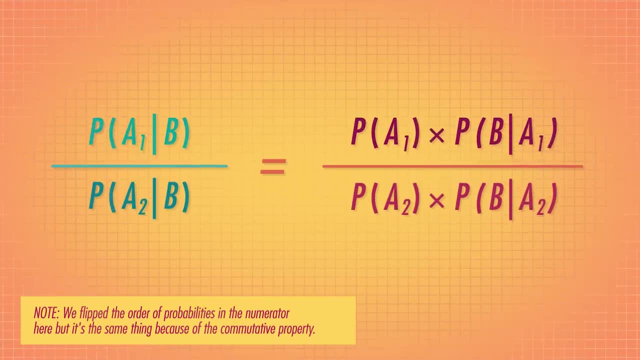 Instead of just calculating the probability that Jordan was a Star Wars fan, given that he'd seen the latest film, we compared the probabilities of the two hypotheses, given that he'd seen the movie. So we're really looking at the ratio of two calculations of Bayes Theorem, because 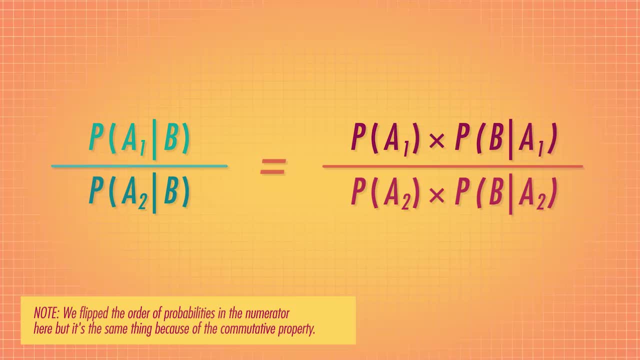 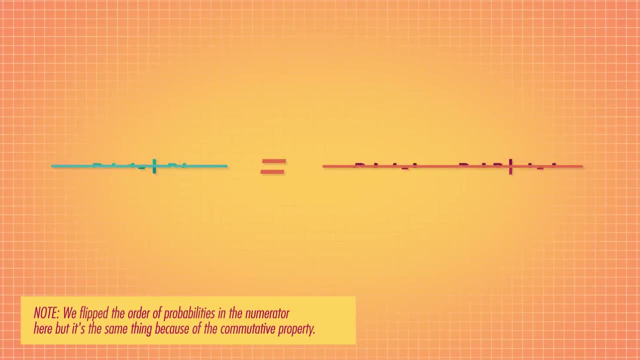 we're comparing two posterior probabilities. Luckily, the probability of having seen the latest film is the probability that Jordan's seen the latest Star Wars movie is the same in both equations, So it cancels out and we end up with this. In Bayesian statistics, these things are called the prior, what you believed before you saw. 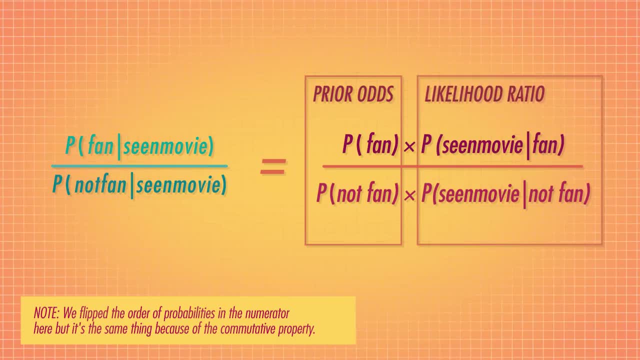 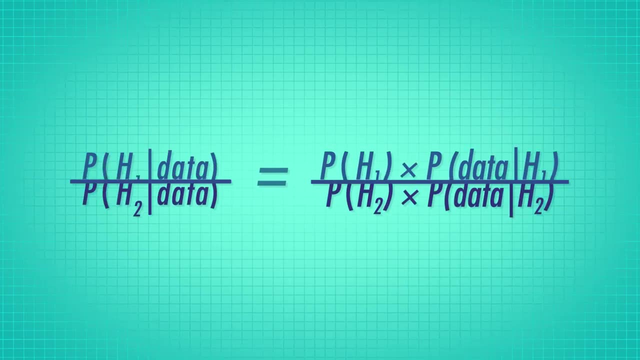 any evidence, the likelihood, a measure of how much your evidence should change your prior beliefs and the posterior, what you believe. after you've seen the evidence In a more general form, we can see that, after we see the data, how likely one hypothesis 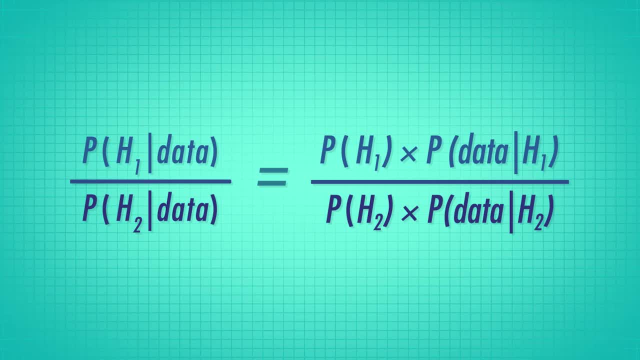 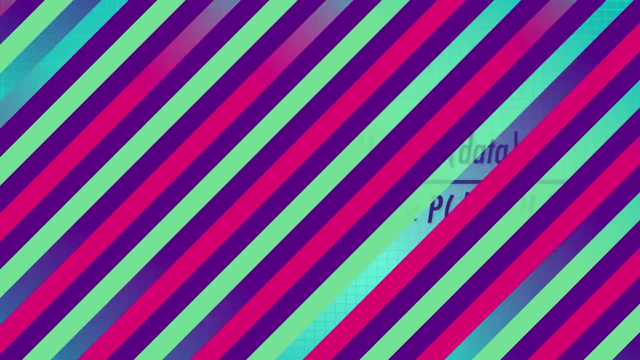 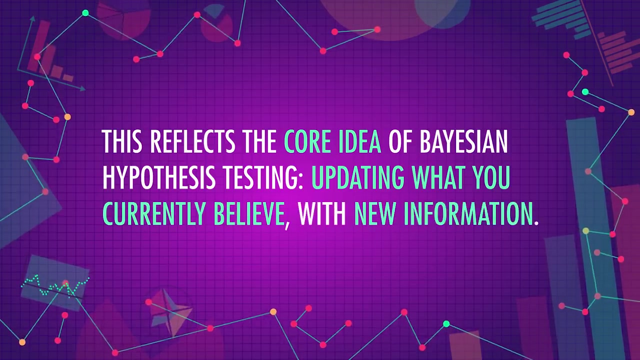 is compared to another is equal to the ratio of how likely we thought these hypotheses were before we got any evidence, adjusted by the evidence with which the data provided us. This reflects the core idea of Bayesian hypothesis testing: updating what you currently believe with new information. 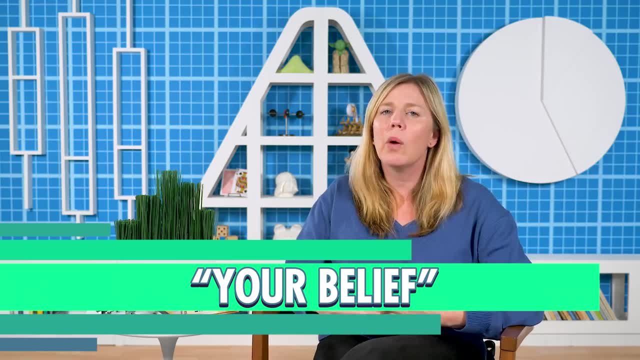 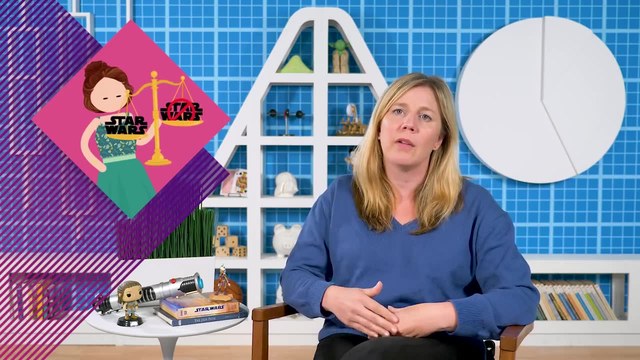 But notice that I said you update your belief Inherently. what we believe is subjective. It depends on who we are and what we've experienced. While Maria initially believed that a Star Wars fan is 1.5 times more likely than a non-fan, 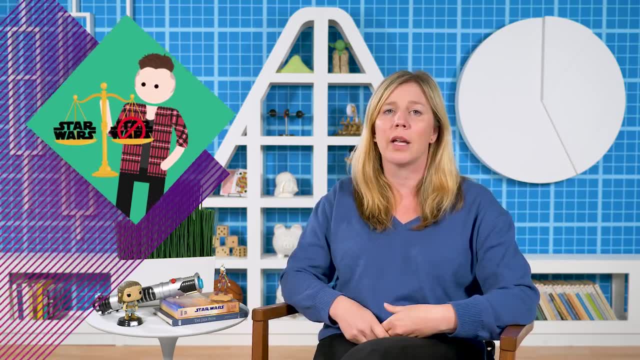 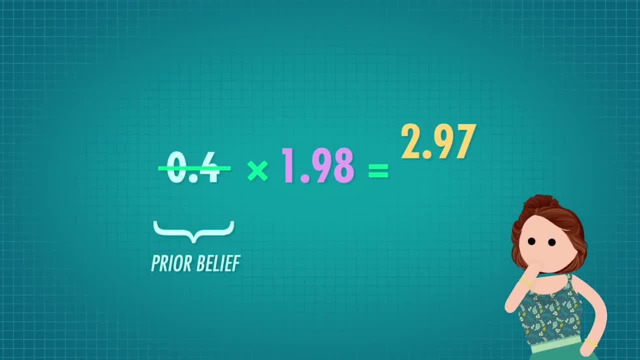 you may believe something else. Like it's just as likely someone is a fan and not a fan, And since this is just a personal belief, it's okay that you and Maria believe something different to begin with, But we use Maria's prior beliefs in our calculations. 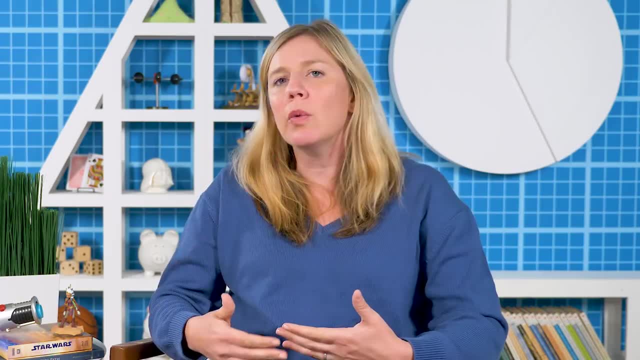 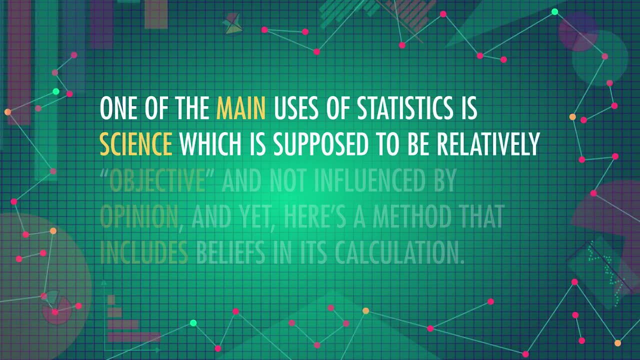 If you were to do the same calculations, you'd come up with a different number, And this is one criticism that Bayesian statistical inference faces. One of the main uses of statistics is science, which is supposed to be relatively objective and not influenced by opinion. 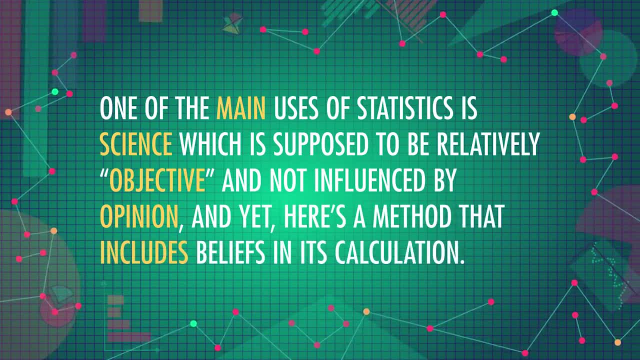 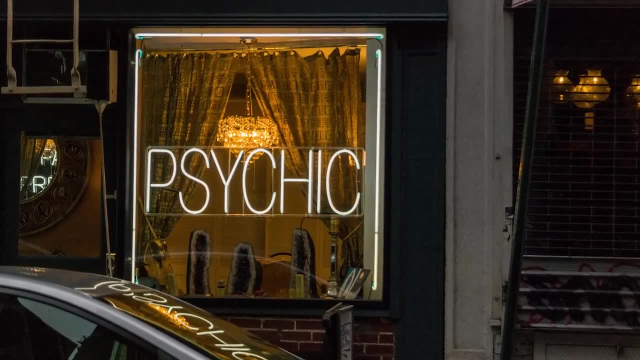 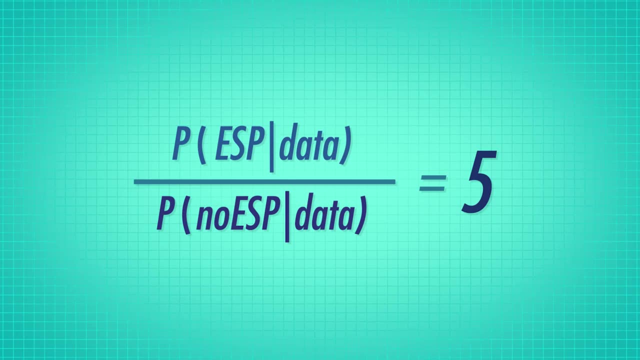 And yet here's a method that includes beliefs in its calculation. For example, say, a scientist bases her conclusion that extrasensory perception exists on the posterior odds of her Bayesian calculation. She concludes from a study that it is five times more likely that ESP exists than it. 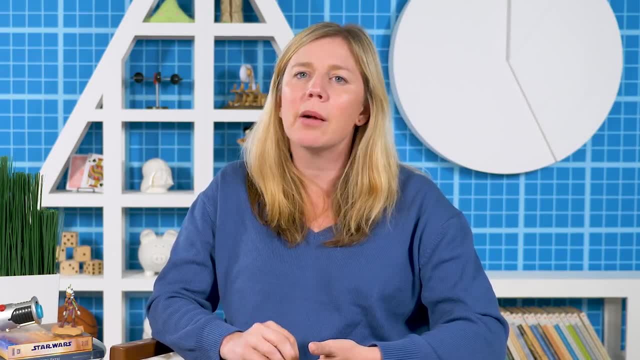 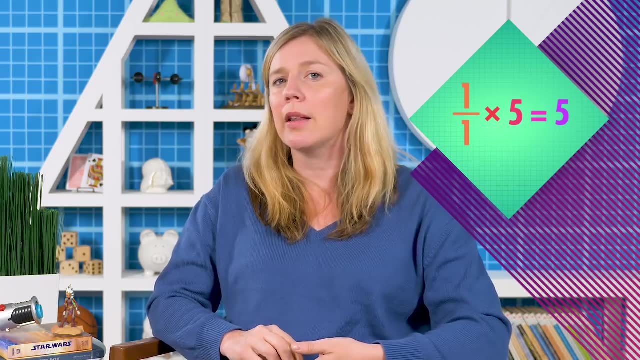 doesn't exist. But upon reading her paper, you find that her prior beliefs about the probability of ESP were way higher than yours. She assumed that it was just as likely that ESP exists as it is that ESP doesn't exist, And that just doesn't seem right to you. 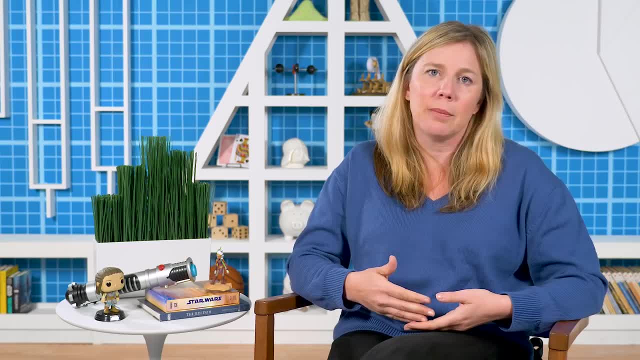 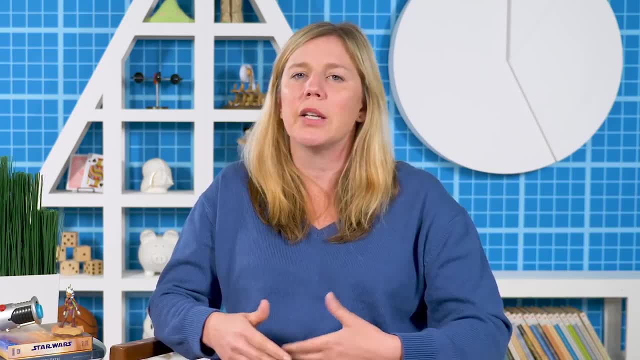 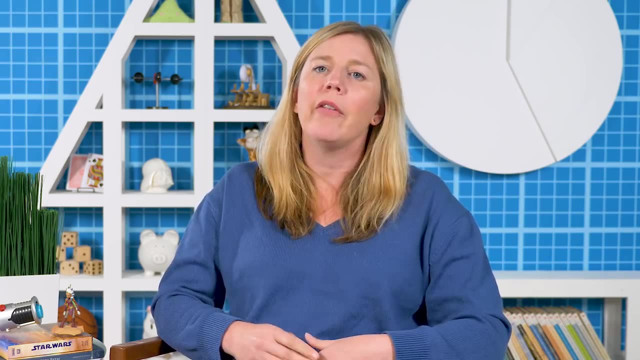 It's just that ESP doesn't exist. But that seems difficult and a bit inefficient. There is a better solution here. Often, studies that use Bayesian calculations will not just report their posterior odds, but also the Bayes factor that they calculated. If you disagreed with a researcher's prior odds, you could use the reported Bayes factor. 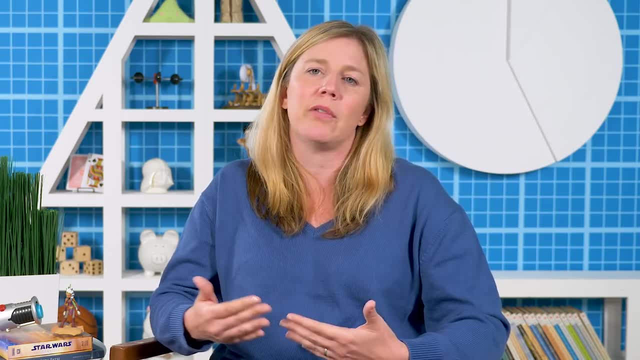 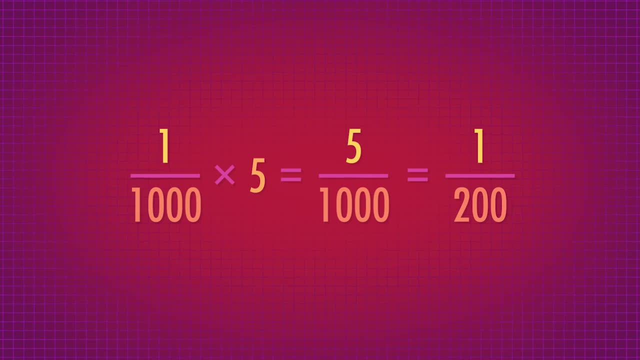 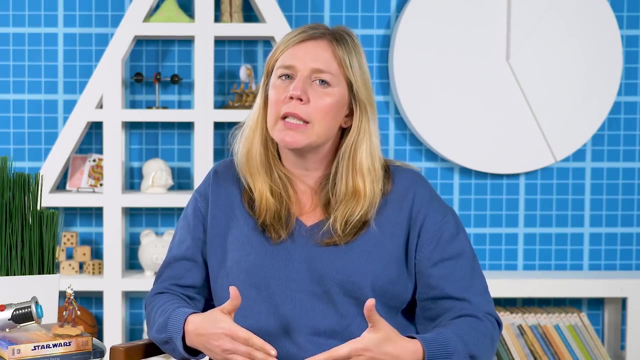 to adjust your own different beliefs about these two specific hypotheses. For example, if you believed that it was one thousand times more likely that ESP doesn't exist, go to the same researchers who reported Bayes factor 5 and adjust your own beliefs, Even though the evidence in the study makes you believe that ESP is more likely than before. 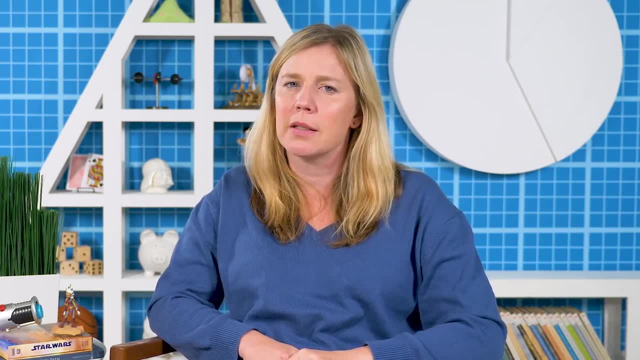 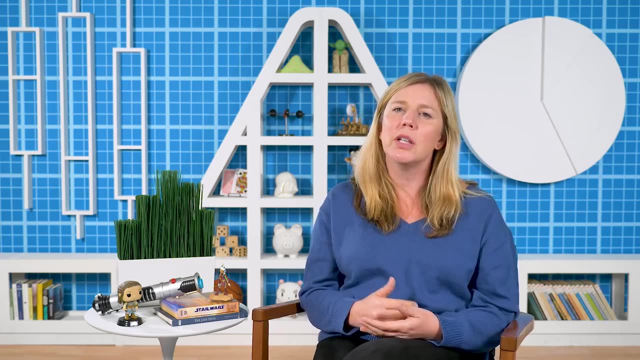 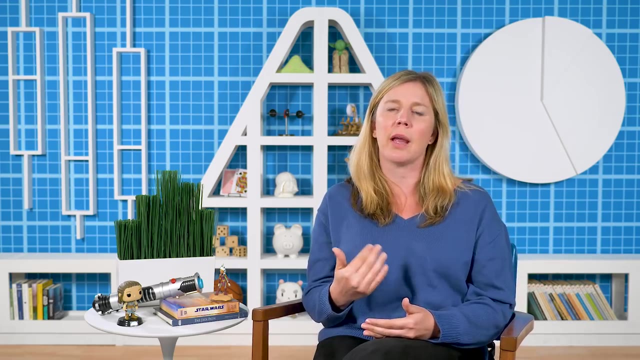 you still think it is relatively unlikely that ESP exists, Even though Bayesian hypothesis testing includes subjective beliefs. the Bayes factor allows you and anyone else to use the evidence from a study or analysis to update whatever your prior beliefs are about the two specified hypotheses. 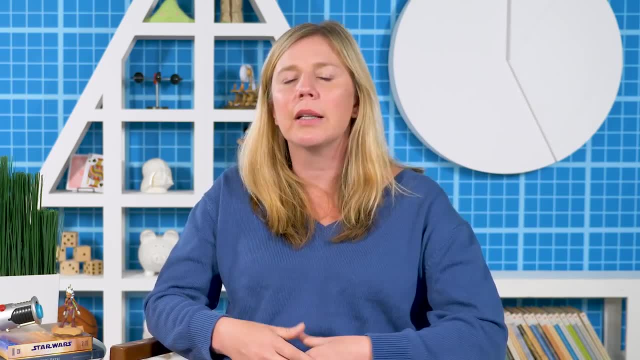 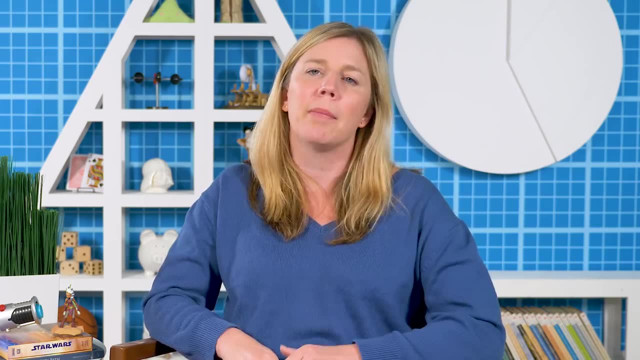 Just like you and the ESP favoring researcher. However, sometimes evidence can lead two people to very different conclusions, But often, unless someone has already decided something has a zero percent probability. when there's sufficient evidence, two people with different prior odds will come to the. 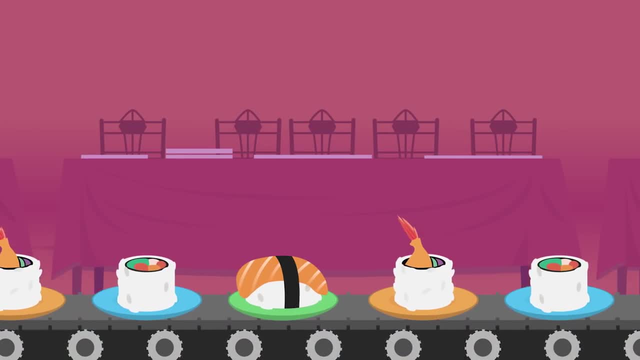 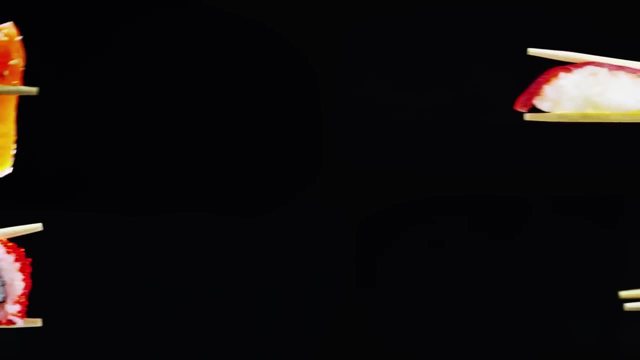 same conclusion. For example, you initially believe that sushi is pretty dangerous and has a high risk of infecting you with parasites, and your coworker thinks that the risk is low to moderate If both of you see your boss and entire team go out to sushi every week for two years and 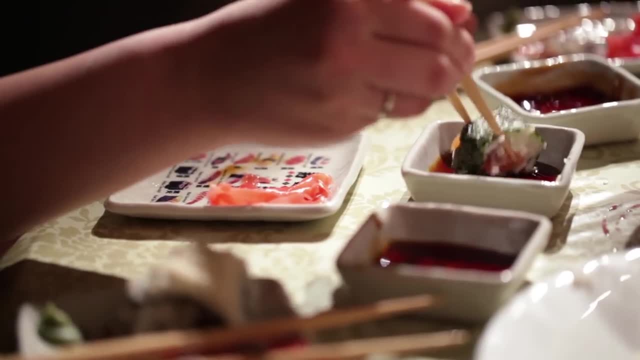 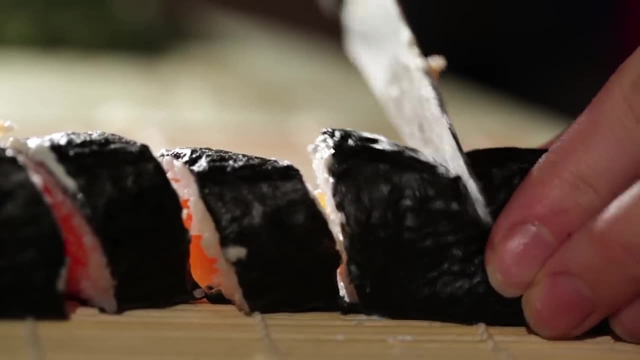 not have any issues with parasites. both of you, despite your initial differences, would probably have updated your beliefs with this new information and concluded that sushi is pretty safe after all. If you had only seen your boss go out to sushi four times without getting a parasite, you 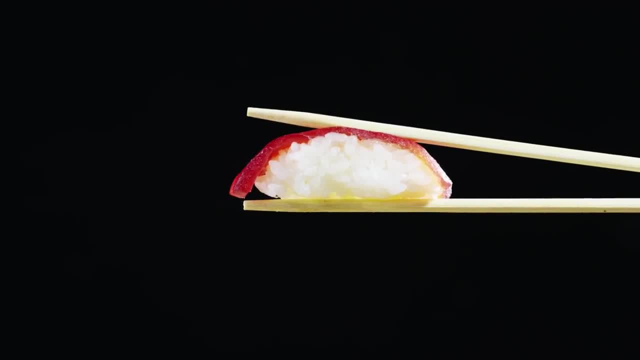 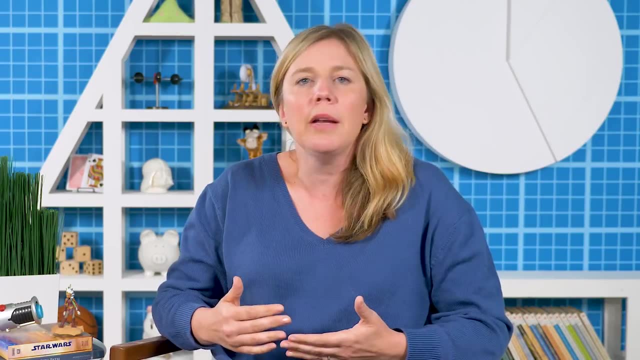 might have come to different conclusions, since that's not as much evidence. You may still think sushi is pretty risky, but that might have been enough evidence to convince your coworker it's safe. Your current beliefs would rely more on your prior beliefs than the new evidence. 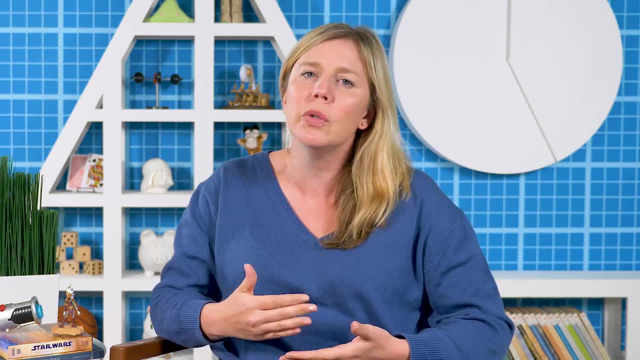 But the huge amount of evidence that you have is not enough evidence to convince your coworker it's safe. But the huge amount of evidence that you have is not enough evidence to convince your coworker it's safe. The evidence provided by a group of healthy coworkers over two years was enough to overwhelm. 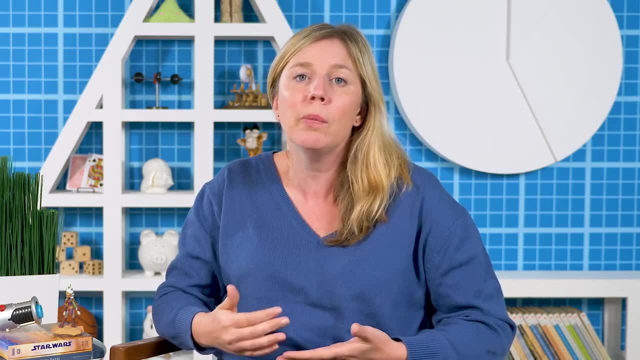 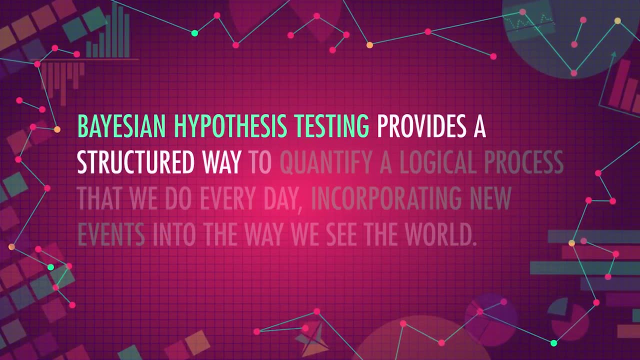 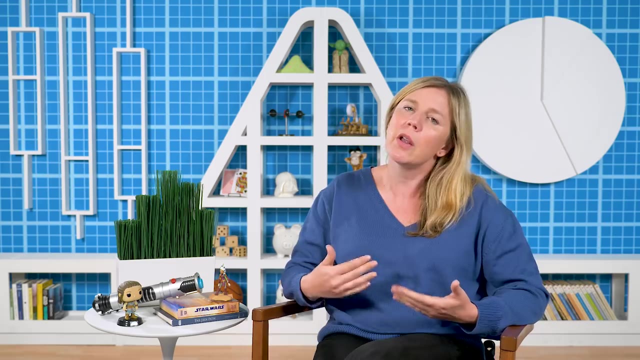 your and your coworker's prior beliefs. so your new posterior beliefs are more affected by the evidence than by your prior beliefs. Bayesian hypothesis testing provides a structured way to quantify a logical process that we do every day, incorporating new events into the way we see the world. 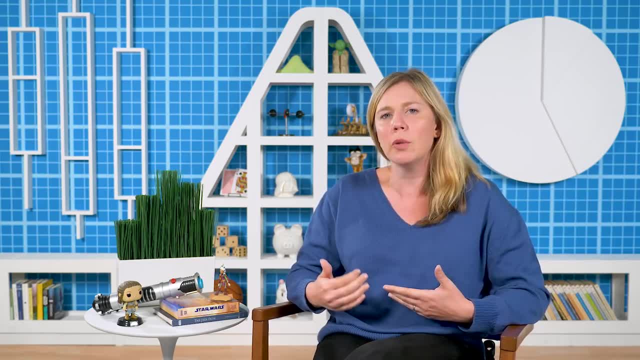 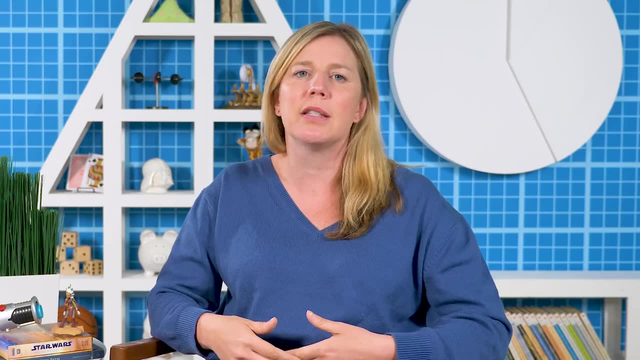 It also provides an explanation, or at least a hypothesis, about why two people can see the same evidence and reach different conclusions In some situations. the logic of Bayesian methods is similar to how we think, naturally, Like a doctor who uses patient symptoms like fever and fatigue to update the prior odds. 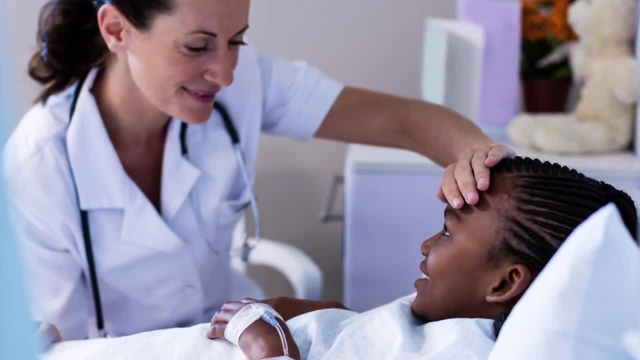 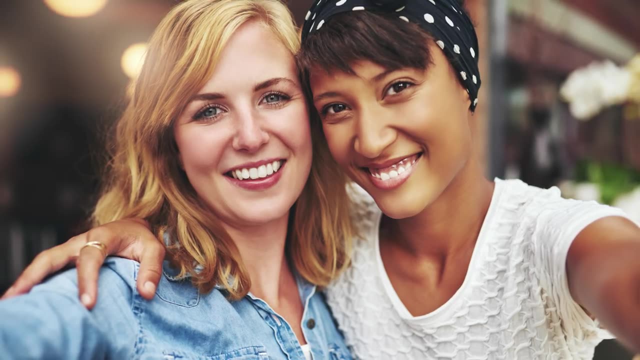 that a patient has the flu compared to a cold, so they can prescribe the correct treatment. Or the way that you updated your belief that your best friend is a kind, caring person by continuously incorporating evidence of their kindness, like covering the cost of your Starbucks when you lost your wallet or helping you move. 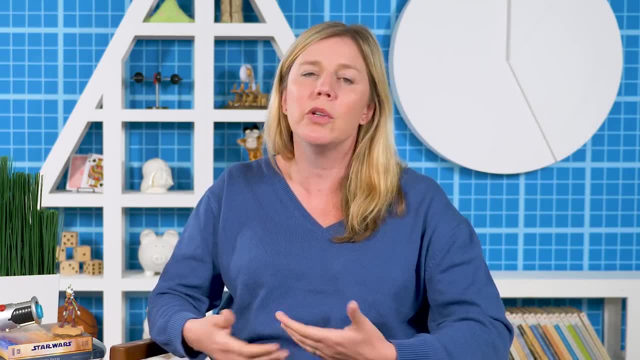 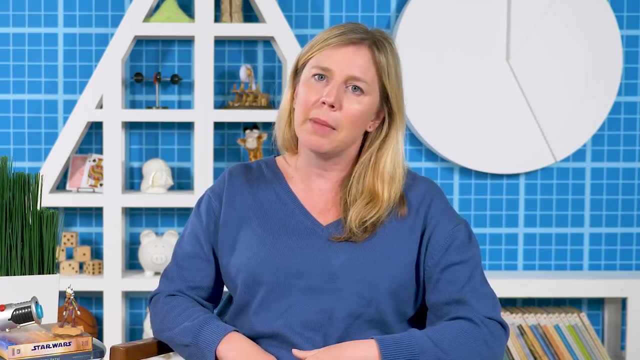 In real life, you don't ignore all previous pieces of evidence you saw as soon as you get a new one, And Bayesian inference allows you to take your new, updated beliefs and update them again. As some Bayesians say, yesterday's posterior, your updated belief is today's prior. the 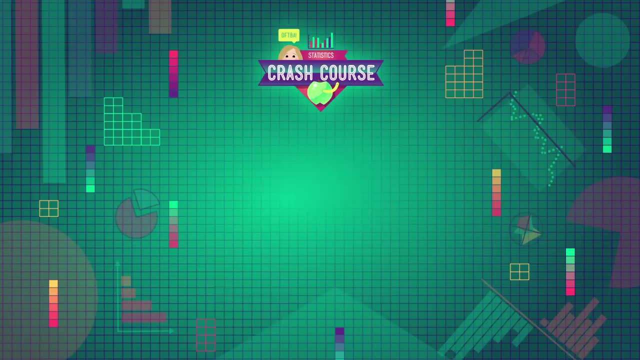 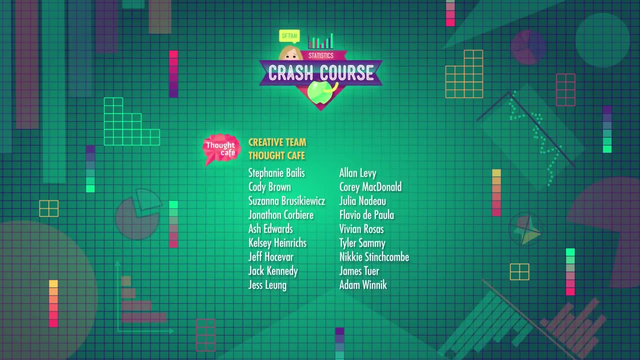 beliefs to be updated. Thanks for watching. I'll see you next time. Crash Course Statistics is filmed in the Chad and Stacey Emigholz Studio in Indianapolis, Indiana, And it's made with the help of all these nice people. Our animation team is Thought Cafe. 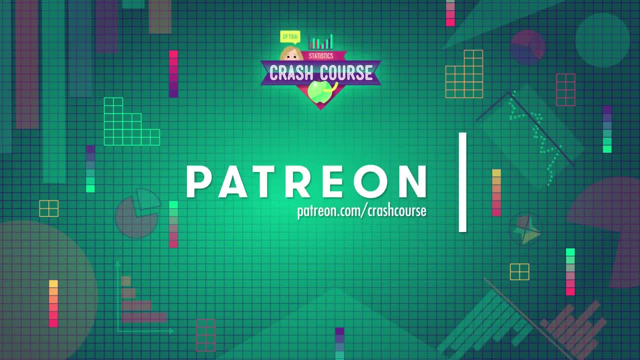 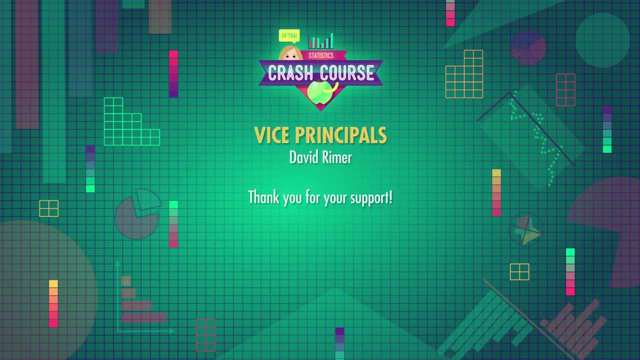 If you'd like to keep Crash Course free for everyone forever, you can support the series at Patreon, A crowdfunding platform that allows you to support the content you love. Thank you to all our patrons for your continued support. Crash Course is a production of Complexly.